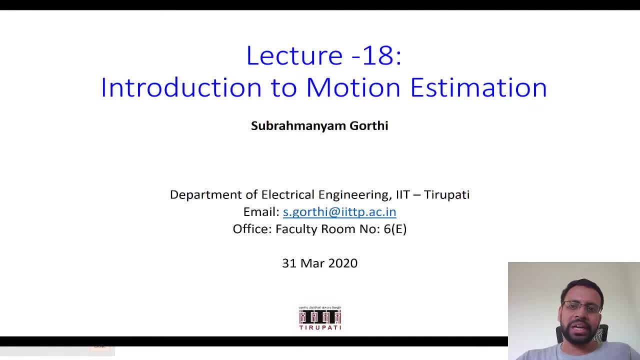 So earlier in our classes we worked. we have finished the key points We started. for example, the continuity of topics were key point detection, key point description, It is followed by key point transformation, key point matching right And then parameter estimation. Now we will be moving into an application mode and the topic would be motion estimation And more specifically, we would be talking about motion estimation using optical flow based approaches. 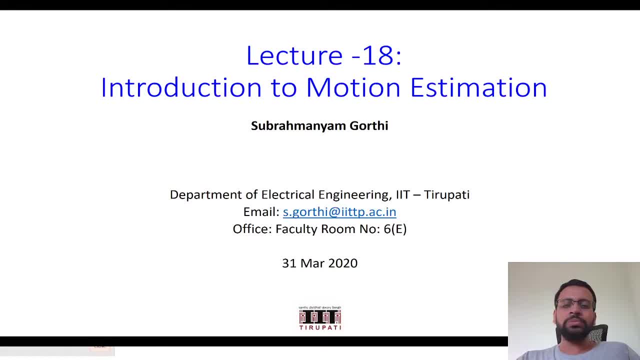 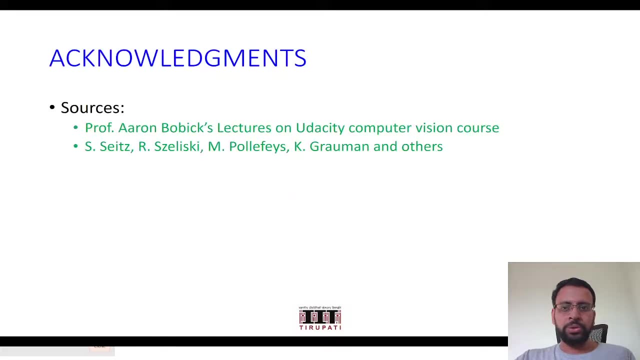 Okay, this lecture would be more focused on more of an introduction to motion estimation And from the next class onwards we will move on to optical flow based methods. Okay, before I go, let me acknowledge here that this is highly inspired. like some of the slides have been adapted based on Professor Arun Bobik's lectures on adaptive motion estimation. 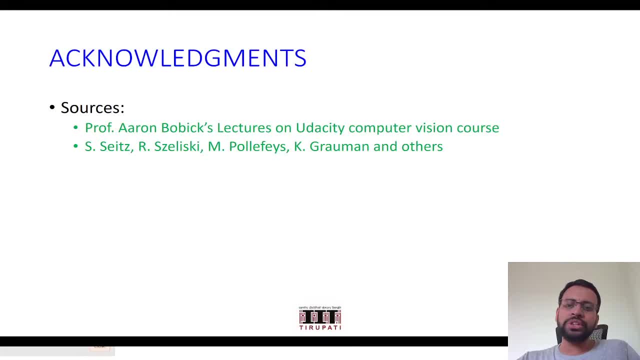 So there are some slides. it is a very good source You could go through. it's a free online course. go through it and then that's also. you can learn a lot from that. Again, Professor Arun Bobik himself would be mentioning that he has adapted slides from various other sources, So some of them are mentioned here. 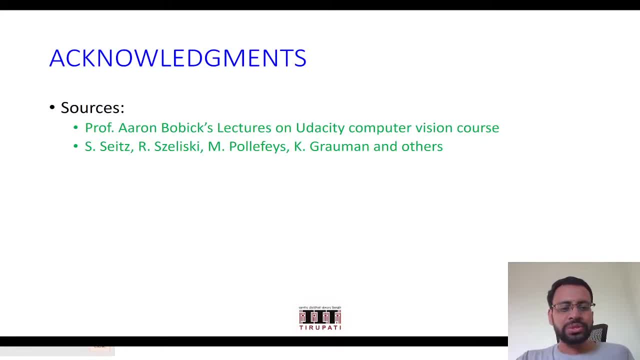 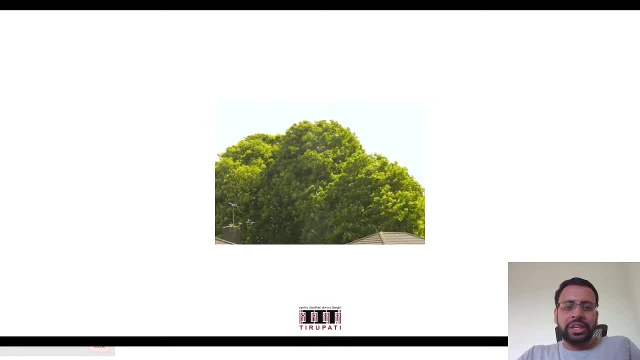 Okay, So once you see any of the course, you can go to that. Okay, So this is what he did. related courses: you will see a lot of the slides in common. yeah, let's start the motion estimation thing. by the way, what do we mean by motion when we look? 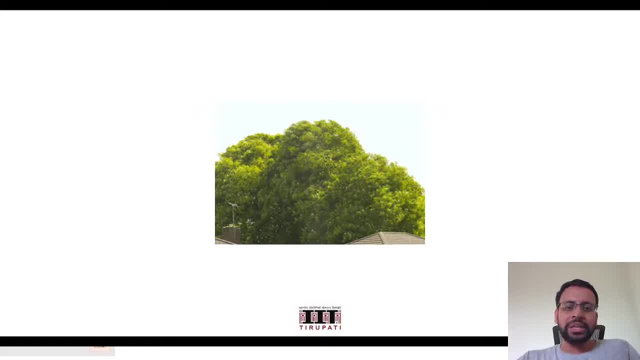 at in terms of a computer vision problem. essentially, that's a question slightly differently posed. is image versus a video, or what we perceive as a motion is essentially, when you are looking at images that have been captured of moving objects that have been captured with a slight delay in time is essentially 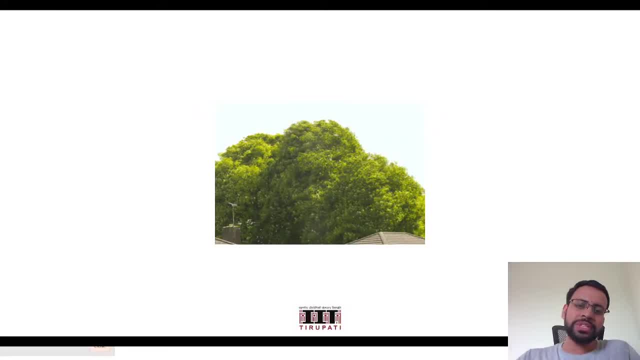 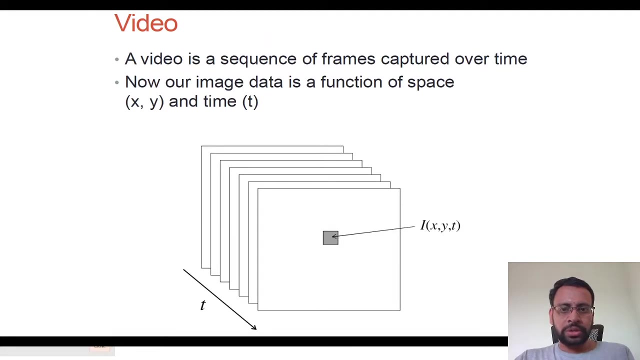 appears like motion. okay. for example, this is one GIF image, okay, which is repeatedly playing, so that you just simply have, when the wind is blowing, how they trees, the leaves of the trees are moving. this is one example. okay, and now, so, as we seen, this is video. we are coming to the video part now. it's nothing but a. 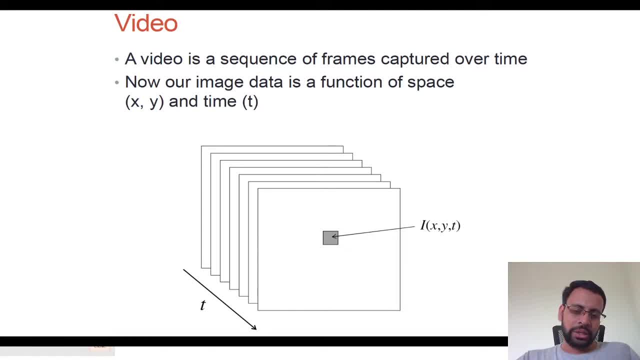 sequence of frames captured over time- the earlier applications we discussed. you have an image which means spatially, you have X and Y. now, in addition to X and Y, you have, over the time, the images captured at different instances of time. that's what I mean. it is between the consecutive frames when we are doing the. 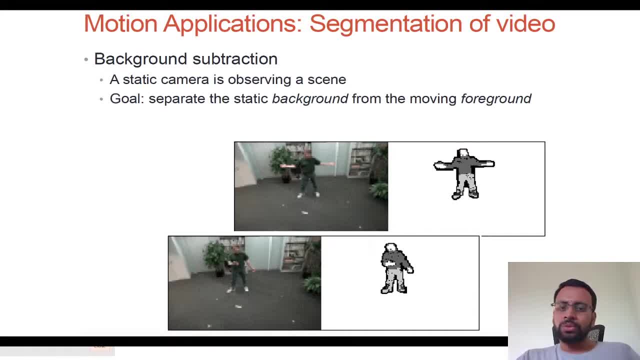 analysis for especially estimating the motion. well, what could be the applications of it? this is again. we will just touch upon a few possible applications of it where you come across this. one of them is, for example, you want to do a background subtraction. you could do it for different purposes. for example, you might be recording you. you'll be. 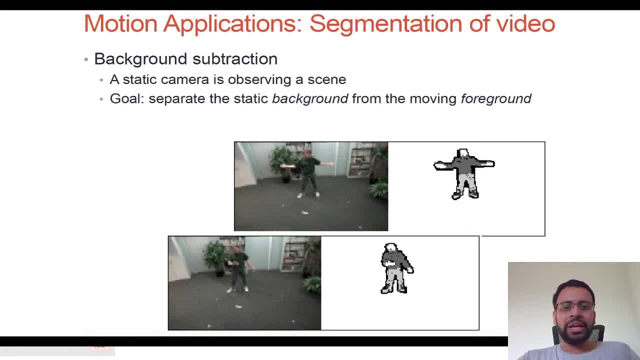 looking at this video itself- whichever is there as a thumbnail there- and then you want to change the background, so you then like to see what are the motions that are there in the video. and then you want to do some background subtraction, so you then would like to see what are the motions that are there in the 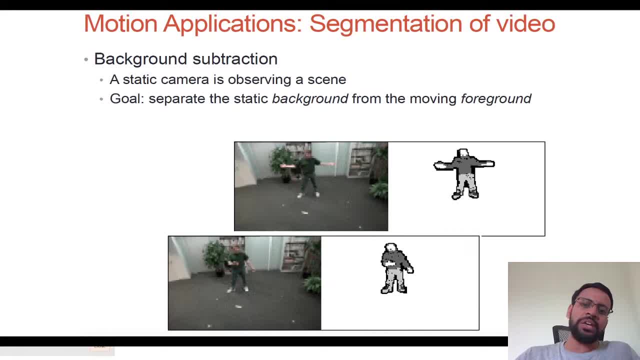 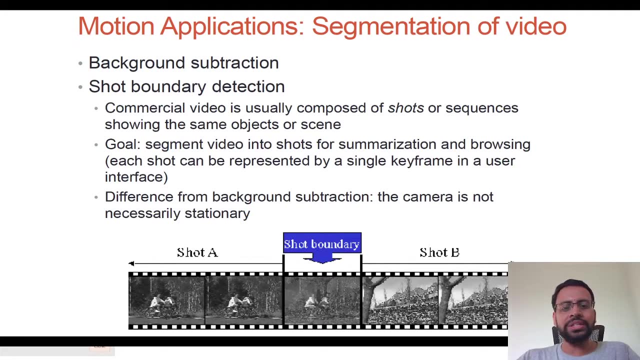 face or in the hands, okay, and then, based on that, you figure out what is the background that is static, and then you could replace with something else. that's one possible application, right, and another application you could think of is segmentation, on finding out the boundaries of different shots that are continuous. for example, let's say, here, in the bottom of the slide, you 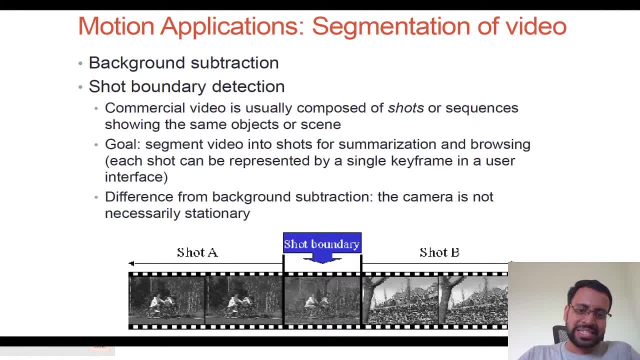 will see an example where there is a sudden change in a sudden transition of the shot. so if you are tracking, you looking at how the pixels have moved from one frame to the other, when you see a sudden movement beyond a particular value threshold, that is where you could figure out that. 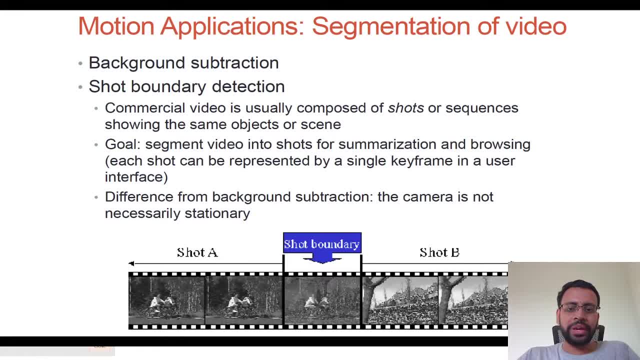 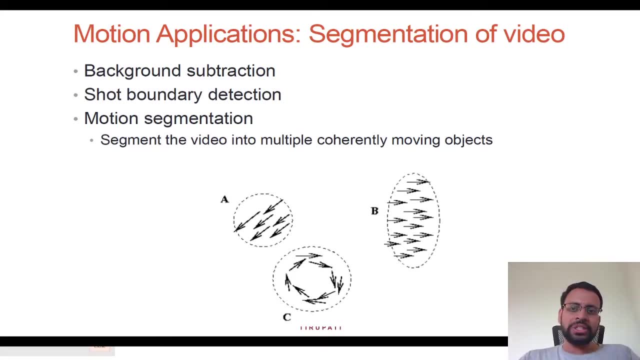 there is a sudden transition here, so that's something one could figure out automatically in a given video sequence for certain purposes. this also you could use. this is one application that you could think of for motion estimation. you and even more practical application is, for example, you would like to detect various 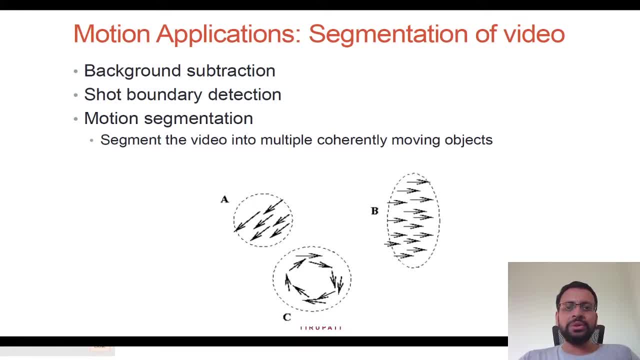 objects that are there in a given video sequence. so how would you do? for example, you could start with an assumption that each object is going to move coherently. say, let's say I am moving my two hands, so you want to get the segmentation of those two hands. so one thing you could assume: 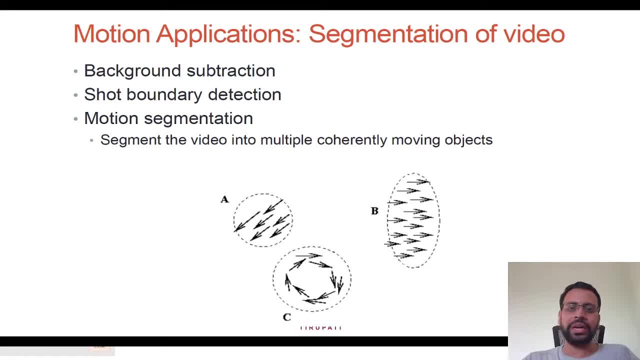 is each hand is moving coherently, or the face is moving coherently, or it could be in any video that you have recorded. there could be multiple vehicles going on and you could make an assumption that each of the vehicle- it's a fair assumption that they are moving coherently, and then you could think of: 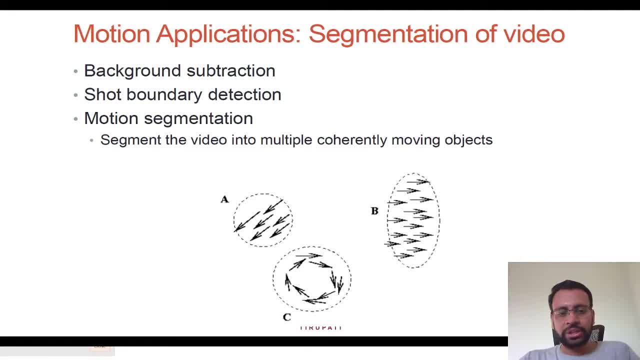 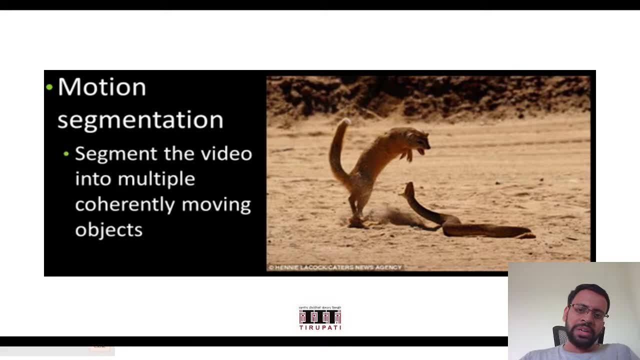 lot of applications derived from that, let's say, counting the number of vehicles, where you could additionally make use of the motion information, and even you could use it for even a static segmentation, let's say you want to. this is one classical example. you find out in lot of places on by how motion 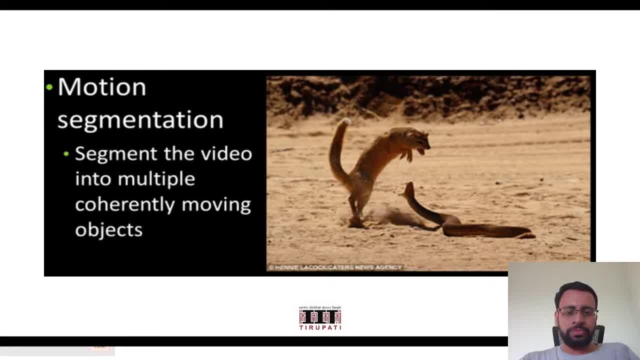 would be useful for even segmenting the objects. so you could see, here the object is, for example, the mongoose and the snake are the ones you would like to find a segmentation. they are very much seamlessly having a very similar texture as the rest of the background. so, for example, there, if you have the motion, if this has been captured, 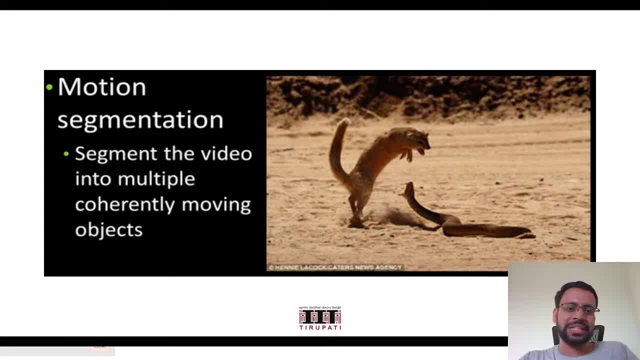 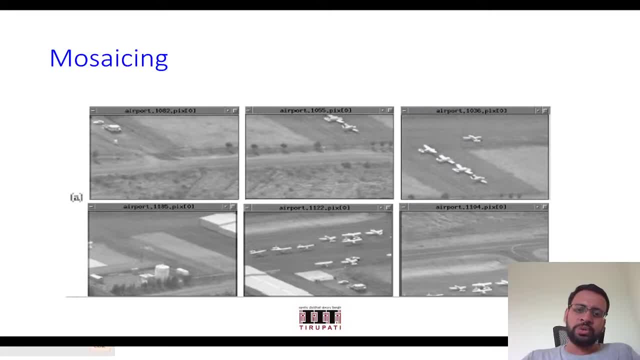 over time and there if you look at the motion of the pixels, that then that is when you could segment those objects right. and another thing is the mosaicing. this again we have seen this application in a different context earlier for key point detection and then matching and other things. again. this example is where 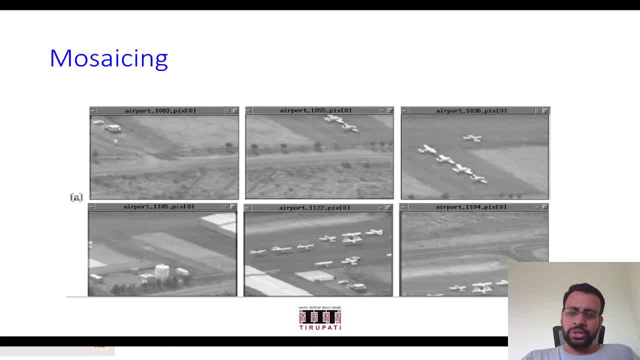 the scene is too large to fit into the lens of your camera zoom and resolution. so what you are doing here is you are. you have captured it. one thing you could by moving your camera. so there is a motion there. if you estimate the motion of your camera, then you could. 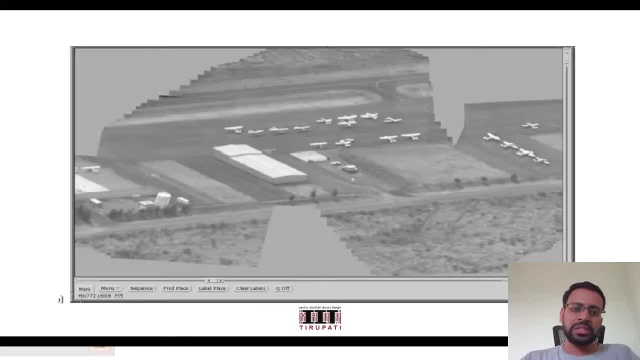 appropriately, stitch them all together, and this is what you could end up. okay, of course, you could have even if there is a movement of, let's say, those flights while you are moving it. with an appropriate model, even you could compensate for the movement of those objects within your scene and 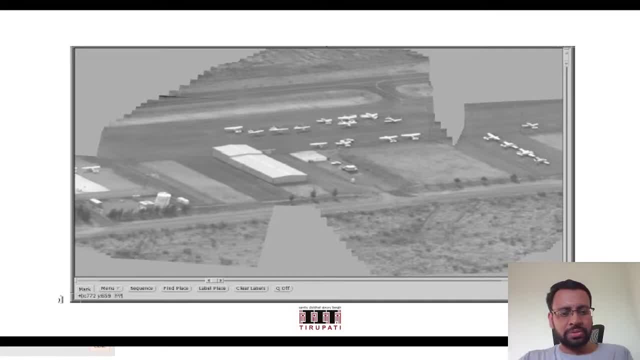 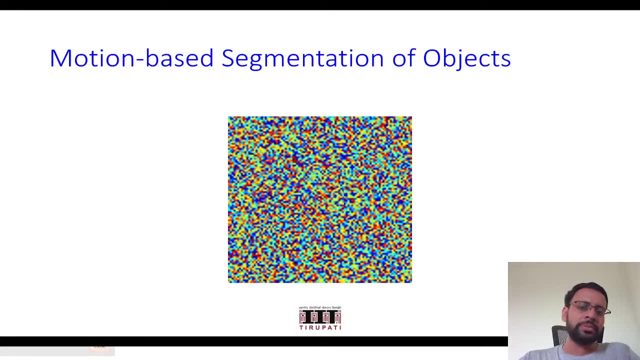 then you could make a nice mosaicing of all those things together. okay, this is another classical example. you will find out in a lot of computer vision. videos is, for example, there, if you have. if you notice closely, there is a moving square within that big square. okay, you can see. it has the same texture. and if you look, 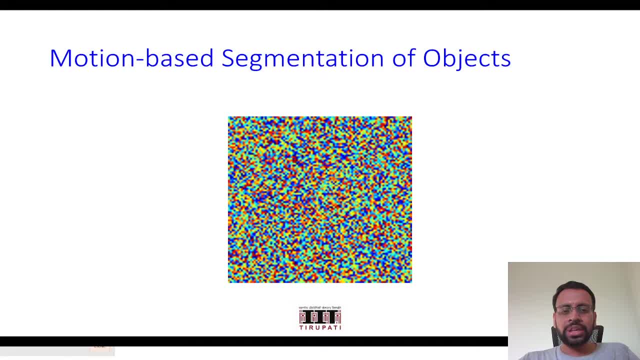 at in a single image of that, in other words, in any frame, you could hardly see that object. but on the contrary, if you have the information of the frames, if you have this over time, that's when you could clearly see in the middle an object moving and you should be able to segment that again. this is a very 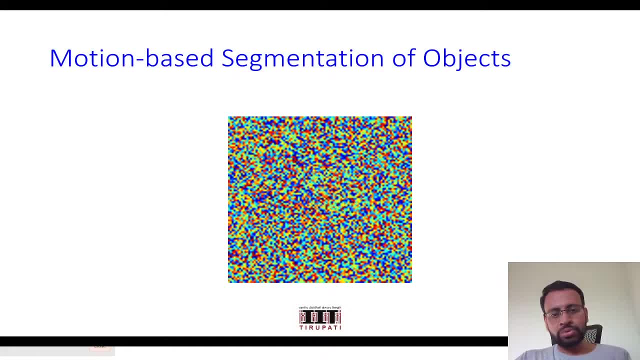 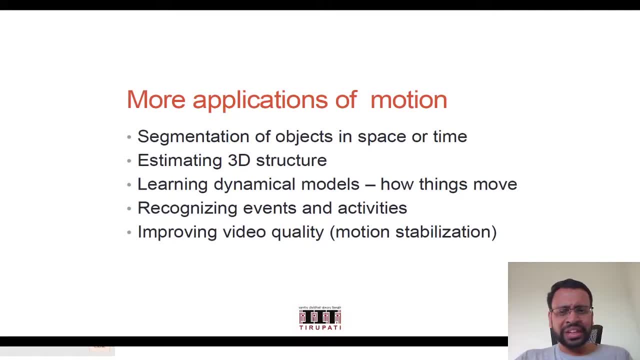 synthetic. Tyler made example to give you the motivation and why this would be required. okay, yeah, this is by no means an exhaustive list of applications of motion estimation, but other things will be: segmentation of objects in space or time, okay, and estimating so, for example, an object is moving, you have segmented. 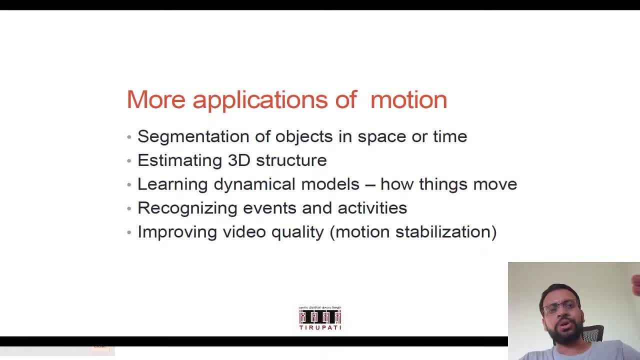 that object in one frame and in the consecutive frame. you want to find out the same object? okay, so this. you could use it as an assuming that the motion is not too high in terms of. you want to find out the same object? okay, so this. you could use it as an assuming that the motion is not too high in terms of. 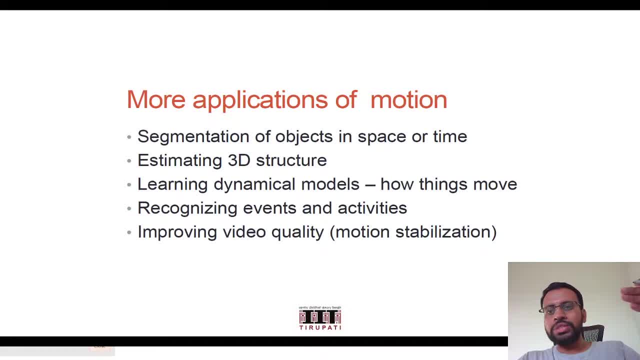 the number of pixels. so what you could do here is you could simply find out this object, you start that as an initialization there, and then you estimate the motion of it. that's how you could get it there, okay. and then the another thing is learning dynamical models how things move. okay, this is for 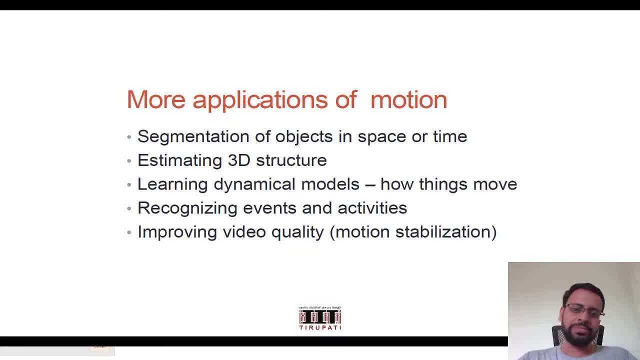 example you want to estimate. for example, one application one of the colleagues is working is cloud estimation to see for for the forecasting of weather forecasting. okay, they are. also the small motion estimation would help to see how the clouds are moving. another thing, for example, there is a recording of video. you have surveillance cameras from that. 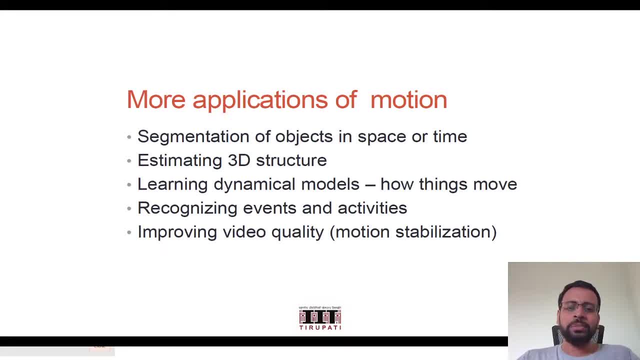 if you want to see and recognize some abnormal activities, again, you need to do how things are moving. so motion estimation would be required and then, while recording something, assume that there is a movement or a zirky thing happening in the camera. so again, if you could appropriately estimate that you. 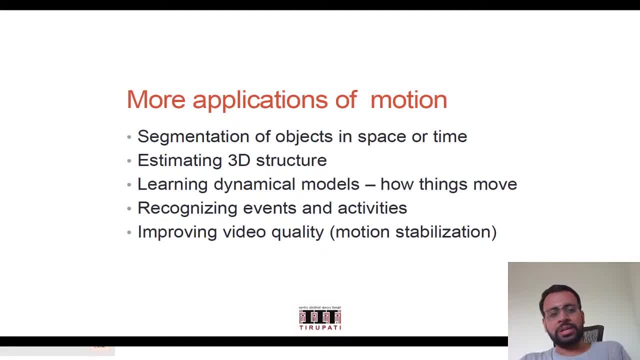 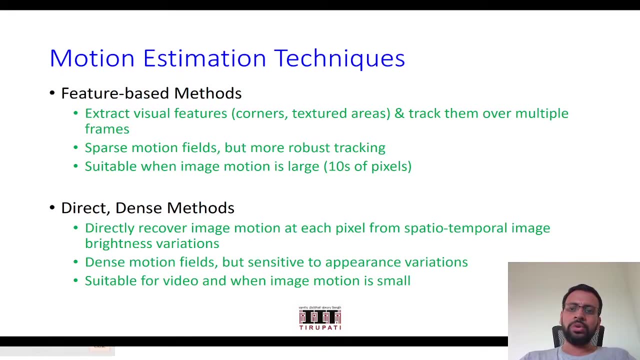 could get an improved video quality. so this is another application that you could think. as I mentioned, by no means this is an exhaustive list. you could see more and more little later as you move on. okay, now we'll come back to the part on how motion estimation techniques can. 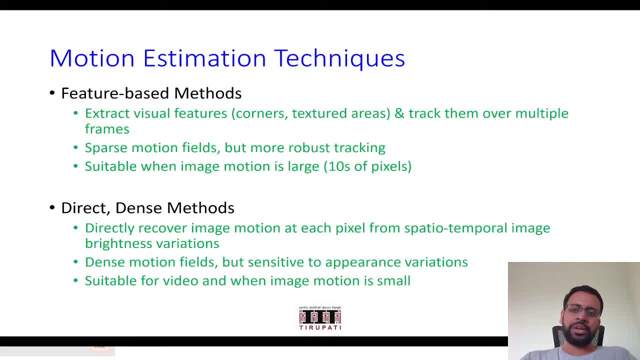 be broadly classified into two categories. okay, one of the first one is feature based methods and the other one is direct dense based methods. what do you mean by feature based methods? for example, instead of using the information that is there in the entire image, what you would do is you would extract some key points within that image, right, and then you 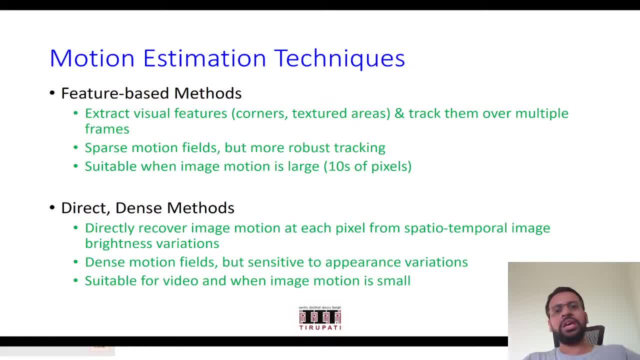 find out. this is again in the another frame. you again extract key points, you try to find a mapping of them and then image transform. so this is exactly what you, you could do with the help of the techniques that we have already- computer vision algorithms that we have discussed in our earlier classes. let's 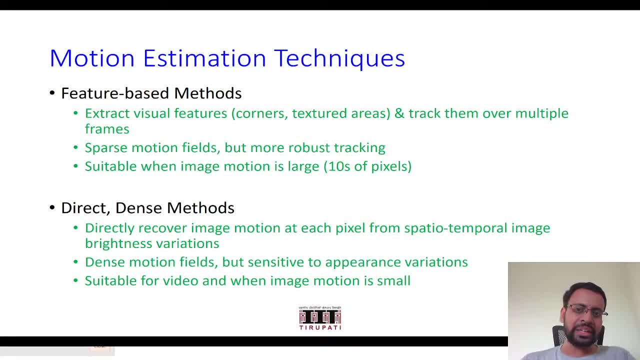 say you start with Harris corner detector, you find out key points, then let's say shift descriptor to encode them, you get the unique signatures of those points and then you use a image transforms to find out the matching between the points and do a parametric fitting of those points. so this is what 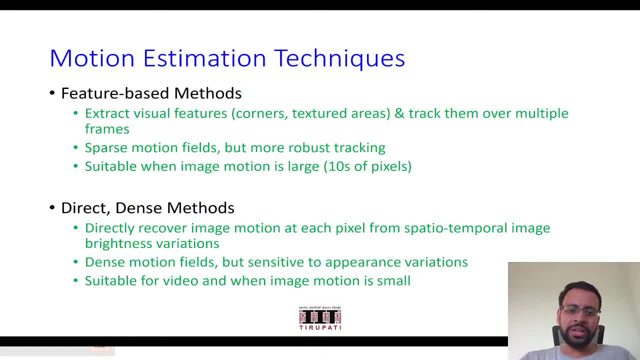 we have done so. the first step is to find out the matching between the points and do a parametric fitting of those points. so this is what we have done. so the first part. we will not be going any further into it and just, and it is what is of. 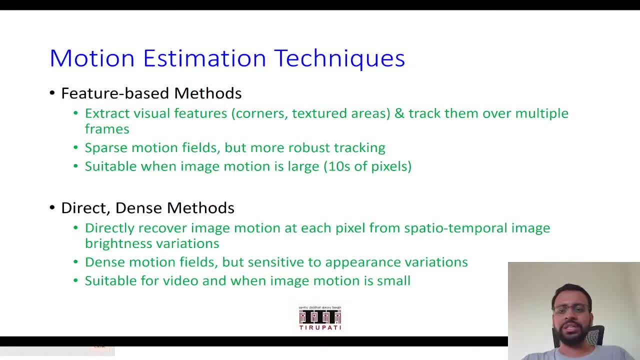 our more interest for the coming lectures, including this lecture, would be the direct dense methods. this would be of our interest for us. by the way, if you compare feature-based methods versus direct dense methods, one thing that you could see is the earlier one, feature-based methods as sparse motion. 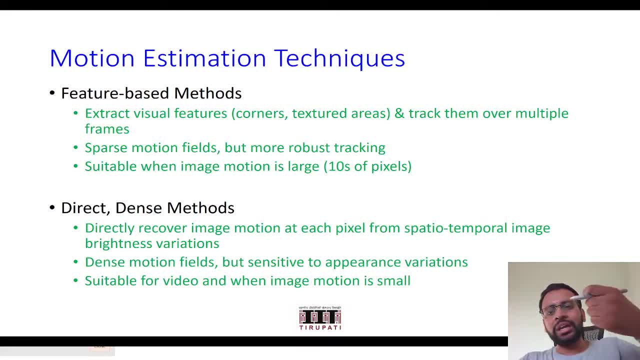 methods right, because you are not getting. you are not looking at how each pixel is moving. rather, what you are looking at is how some key points are moving there. okay, so that that is how you are not getting it at every pixel, but, on the contrary, it has an advantage as well. this is very robust to tracking. 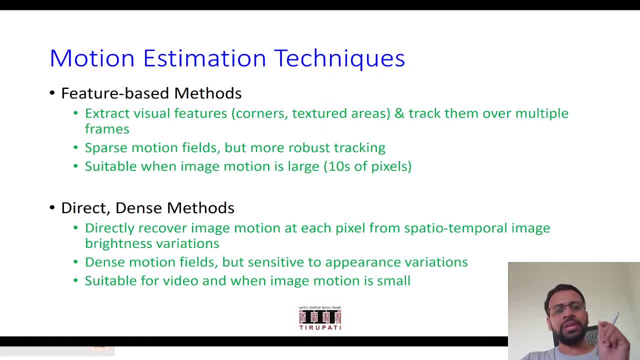 because you have seen earlier that these key points are very reliable to detect, and so that's the advantage it comes up with. then you, you, basically there is suitable. these are particularly so. motion is very large, some tens of pixels. motion is there. you would see shortly in these optical. 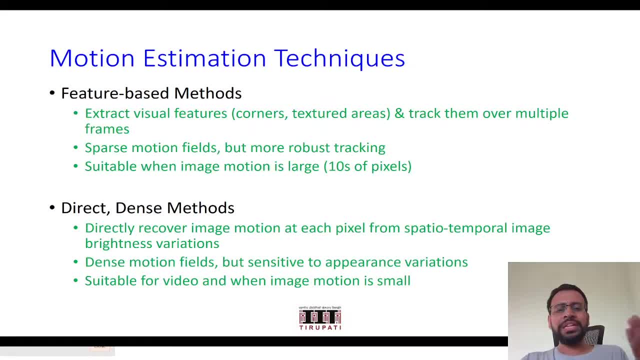 flow based methods will be of sub pixel accuracy and hardly two, three pixels around that if there is a motion that it could effectively do it. so that's why you go for feature based methods. okay, usually when the image motion from one frame to the consecutive frame is very high, which is of 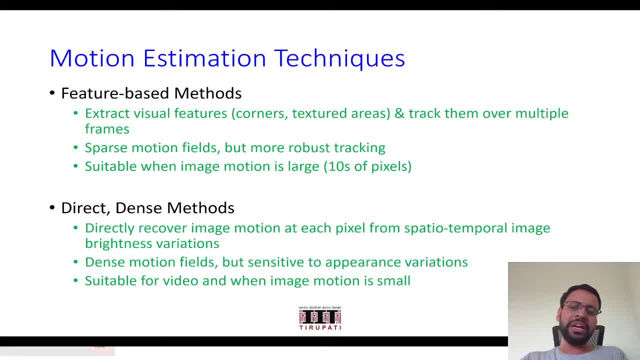 the order of tens of pixels. okay, on the contrary, the direct dense methods is: you call it as dense because you are going to get the motion estimation at every pixel, so the estimation of this motion is very dense, so you call it as dense methods. so, and they recover image motion at each pixel from. 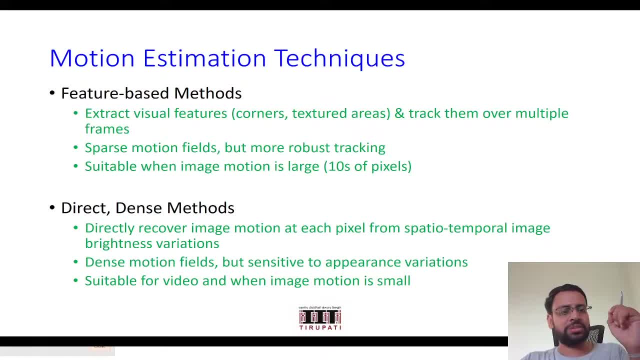 spatio, temporal, image, brightness variations. okay, so you call it spatio because it is an x, x, y, an image. you call it temporal, you call it spatial because you have a t, tv, instances of t, t plus 1, t plus 2 and so on, and your mapping would be you. 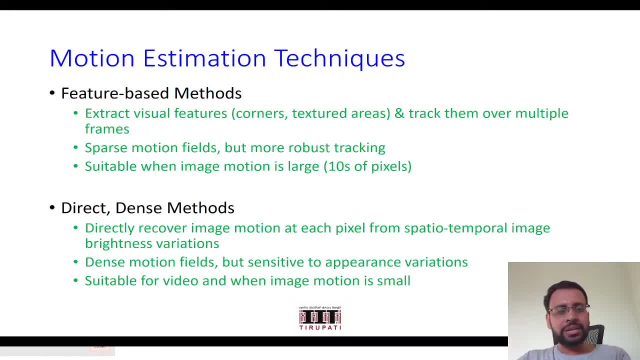 will see in the next video lecture that this mapping would be essentially based on the brightness intensity values of the pixel. so this is essentially based on spatio, temporal image brightness variations. okay, as we discussed, this gives dense motion fields. okay, but they are sensitive to appearance variations. so if there are small changes in the appearance, they're stretching or contract. 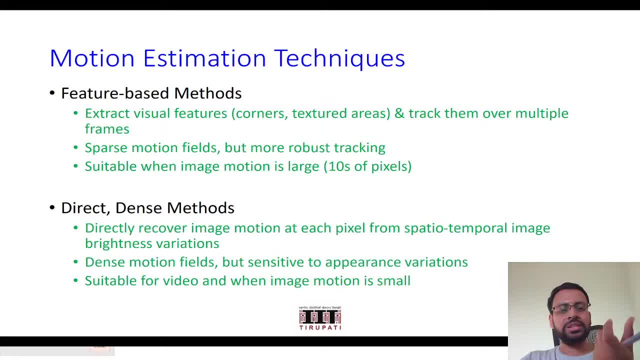 contracting in small regions also. since this is dense, this will be able to capture those things, and this is suitable for video when your image motion is small. so sub pixel accuracies if you want to get it's just moving around that pixel. that is when these are very much suitable, okay. 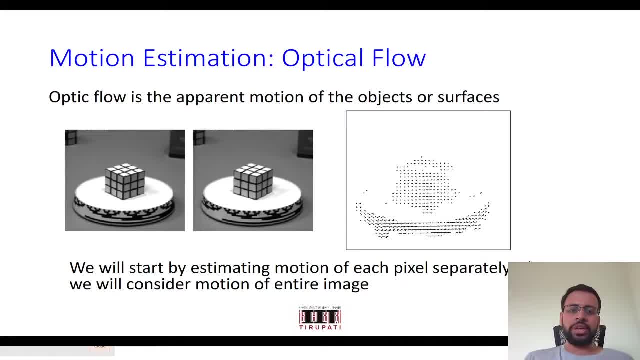 this is another example for motion estimation. okay, particularly, this is another example for moving around the light Bridge. so if you want it, if you want there to see an object of a particular kind of tension, then on where the distance from the朋友 here you would see a inlet, very long distance interval, which is the one being as ambitious. 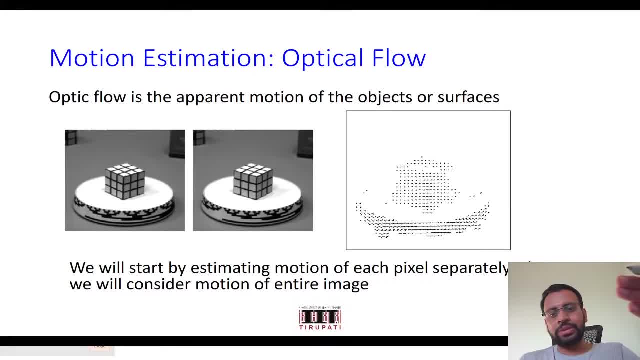 pequeño spoonfuls rest. so, as I already made the same, I just wanted to show the definition, yes, an example. so how you, how you actually would definitely have the technique that you are going to learn over and over again. okay, so you just have fat area right here. so you, 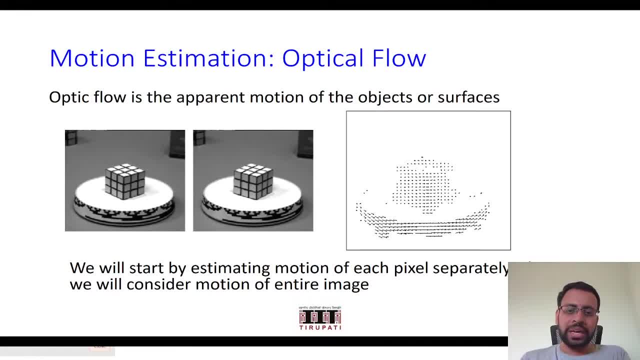 would have a says: create custody widths and so on and so on and so forth, all of these images. you would overall have 30 different undergo options of how it would одноanalyze the information you're upto and that's all. folks吹 is, for example, again from one of the papers, very long back papers. so there is a dice which has been 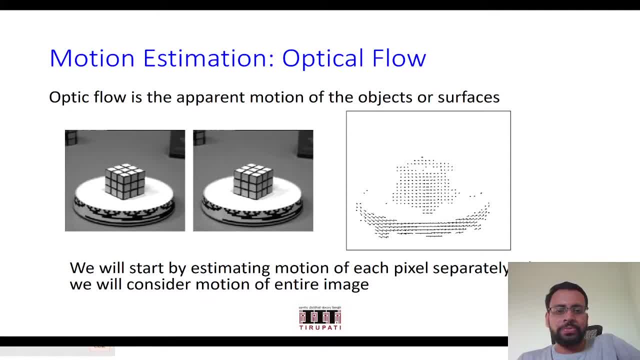 kept on a rolling disc so that's rotating, and if you find out the optical flow which should give you, at every pixel, the motion estimation, you would see that in the regions that are away from, say, like where there is a uniform region, you won't get anything because apparently the brightness would 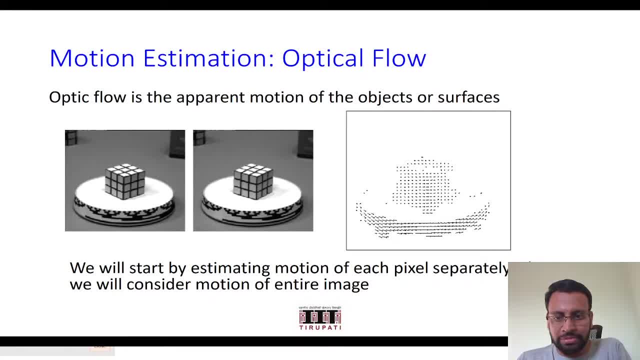 remain the same. because if you assume, i don't know, but that platform which looks like a cake, okay, that platform, for example, is white. there is no textural difference there, so you hardly see anything there, any difference there. so it gives as if the motion field is zero and 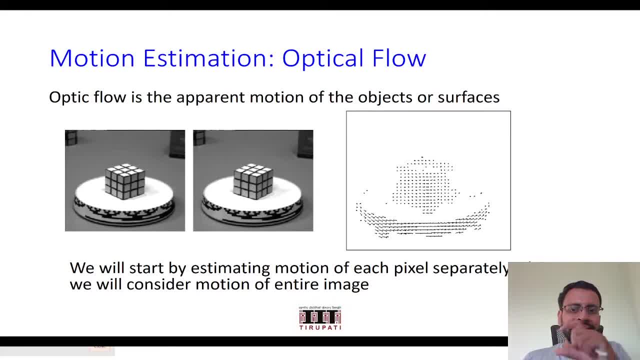 yeah, there is some textural variations on the outer side of the rotating part and another interesting thing that you could observe here is those for that 3d object, for those pixels which are closer to you there you see the motion large, and those that are far away on that rotating disk you will see the motion. 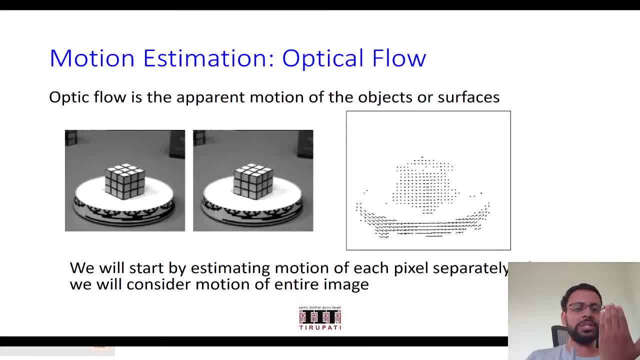 small. this makes sense because whenever the object is closer in that frame, even a small movement there in 2d it appears as a large movement compared to those pixels that are far away, right? so this is one example of motion estimation using optical flow, right? so this essentially uses the entire image and is 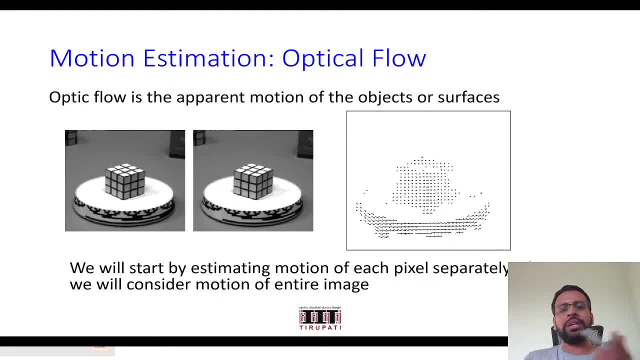 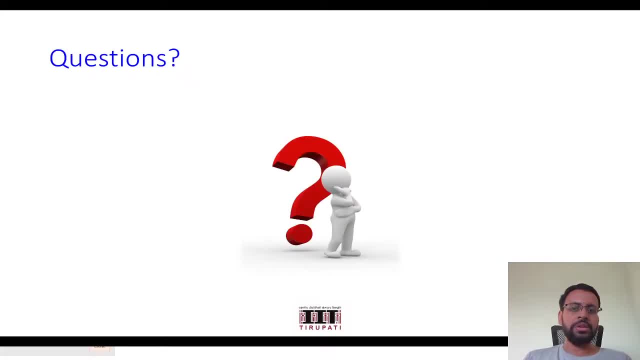 good for those cases where you expect sub pixel motion or motion of few pixels, not tens of pixels, and other things. okay, yeah, this is that's all the introduction to what motion estimation is, and in the next lecture, you would see, we will, you will, we will start discussing about optical flow methods. okay, yeah, hope the concepts.